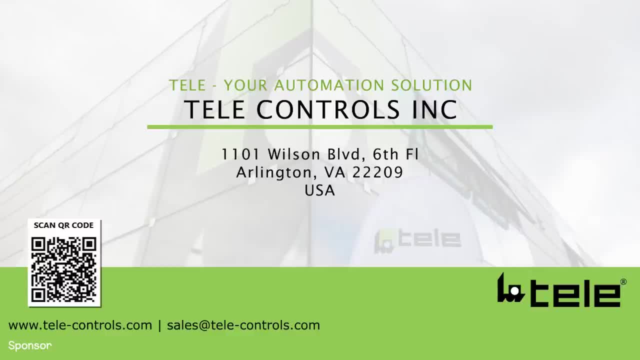 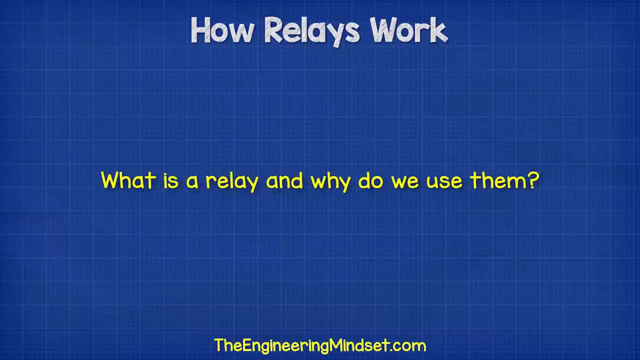 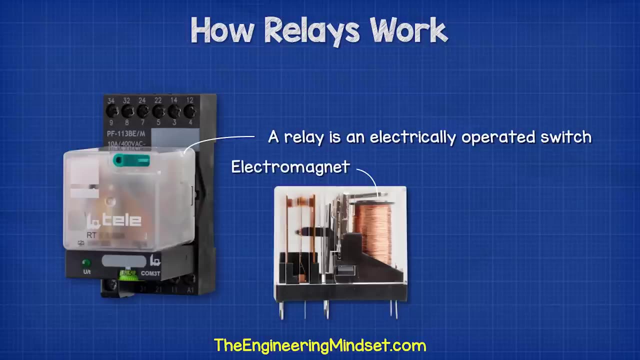 telecontrolscom or through LinkedIn to receive your free relay configuration cheat sheet. For more information, see the link in the video description down below. A relay is an electrically operated switch. Traditionally, relays use an electromagnet to mechanically operate the switch. However, 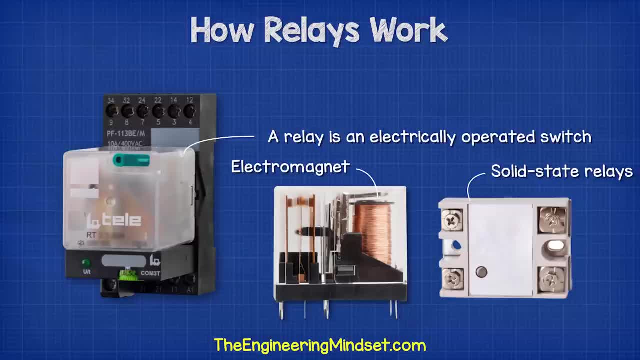 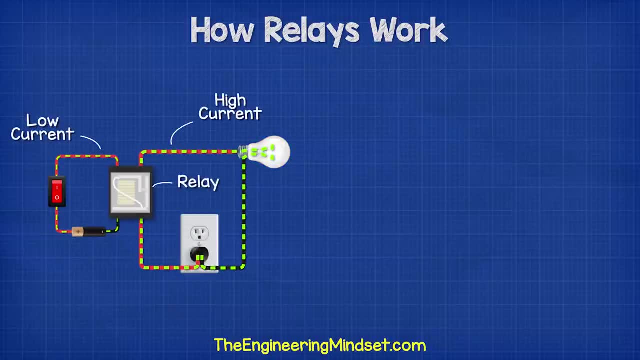 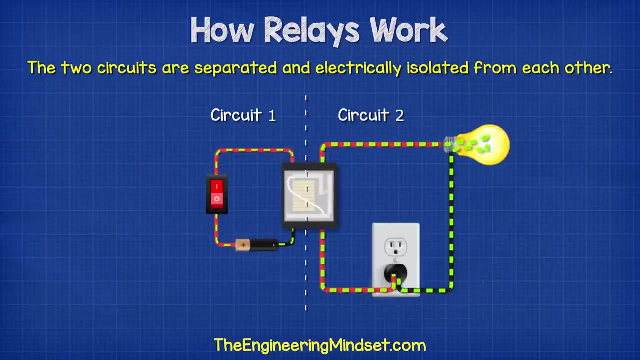 newer versions will use electronics such as solid-state relays. Relays are used where it is necessary to control a circuit using a low-power signal or where several circuits must be controlled by one signal. Relays ensure complete electrical isolation between the controlling and the controlled circuits. 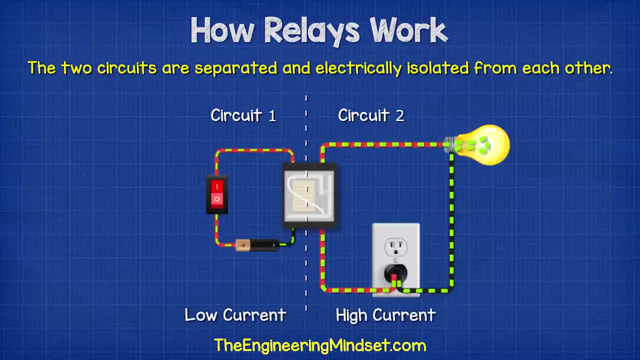 Relays are often used in circuits to reduce the current that flows through the primary control switch. A relatively low-amperage switch, timer or sensor can be used to turn a much higher capacity load on and off. We'll see examples of this a little later in the. 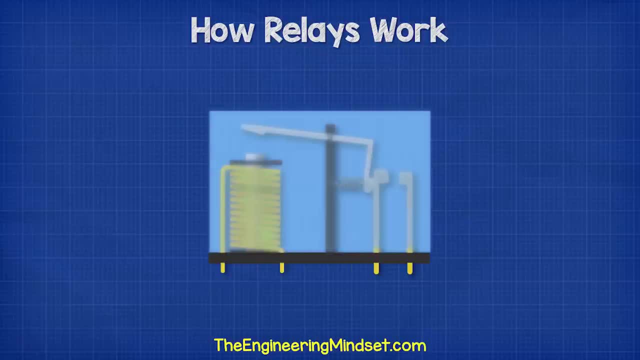 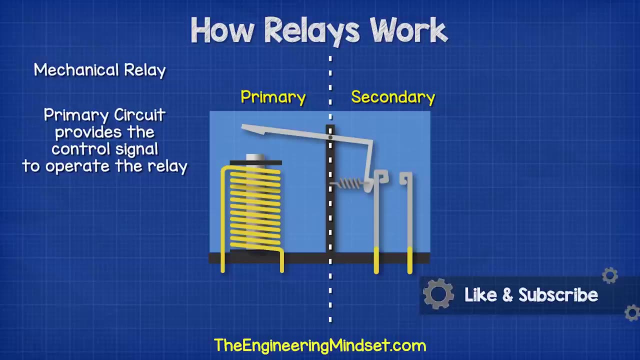 video. There are two main circuits in the relay: the primary side and the secondary side. The primary circuit provides the control signal to operate the relay. The relay is also used to control the circuit. The relay is also used to control the circuit in the relay- The primary. 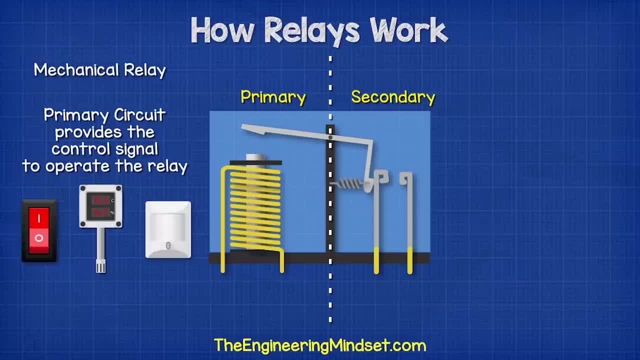 circuit is used to control the circuit in the relay. The primary circuit is used to control the circuit in the relay. This could be controlled by a manual switch, a thermostat or some other type of sensor. The primary circuit is generally connected to a low-voltage DC supply. The secondary 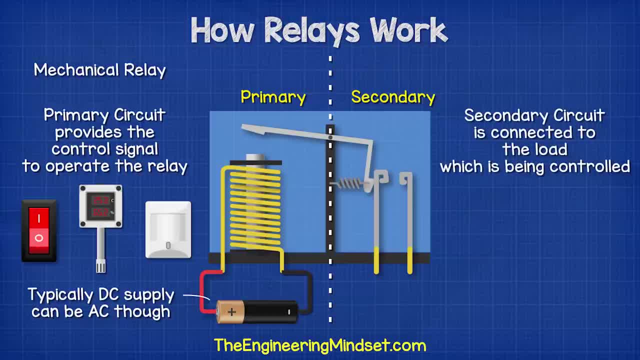 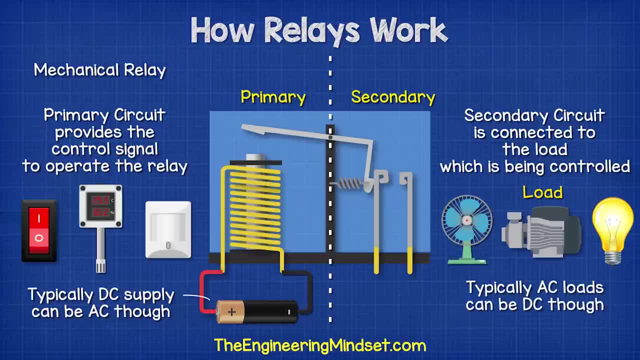 circuit is the circuit which contains the load which needs to be switched and controlled. When we talk about a load, we mean any device that will consume electricity, such as a fan, a pump, a compressor or even a light bulb. On the primary side, we find an electro-magnetic. 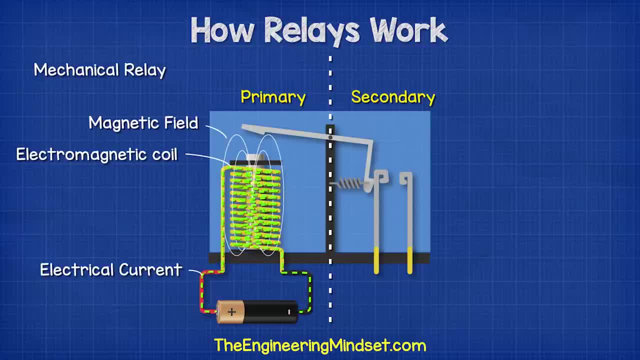 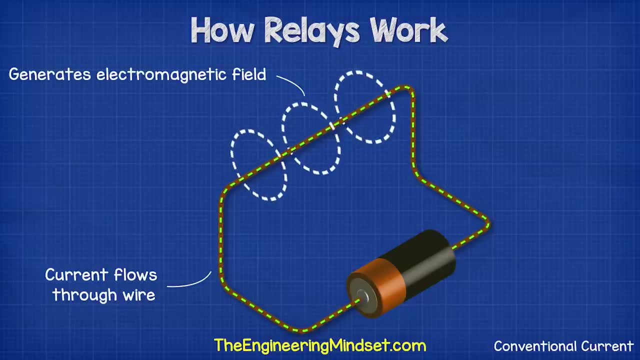 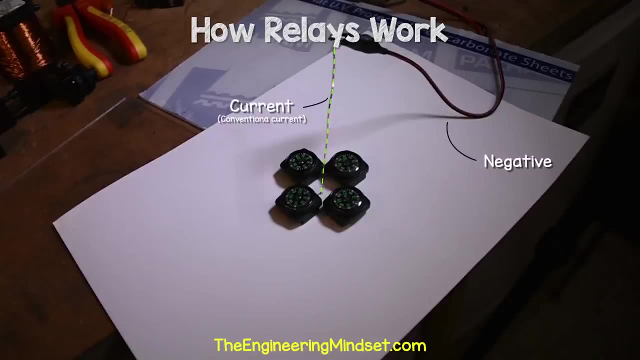 coil. This is the coil of wire which generates a magnetic field when current passes through it. When electricity passes through a wire, it creates an electro-magnetic field. We can see that by placing compasses around the wire. When we pass a current through the wire, the 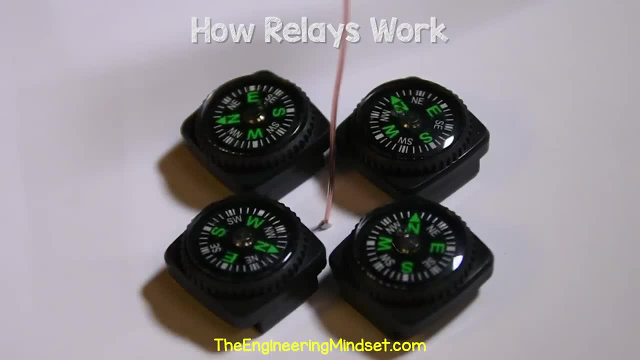 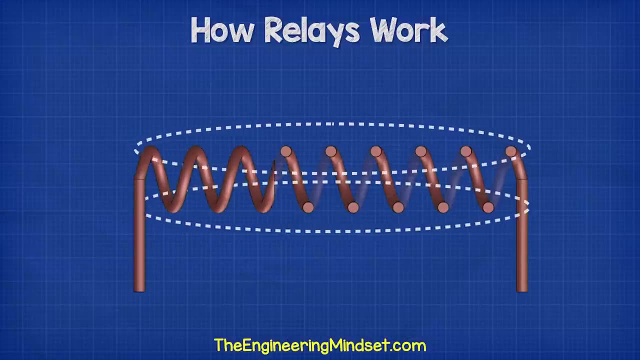 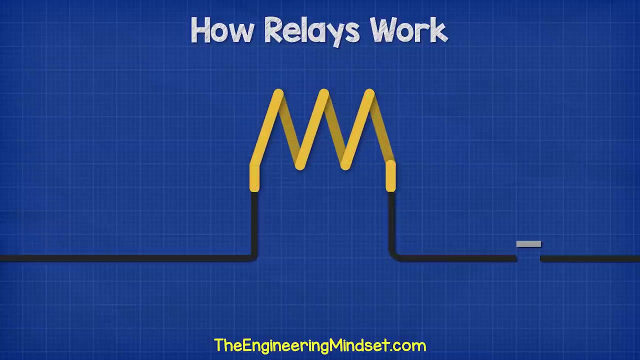 compasses change direction to align with the electro-magnetic field. When we wrap the wire into a coil, the magnetic field of each wire combines together to form a larger, stronger magnetic field. We can control this magnetic field by simply controlling the current. 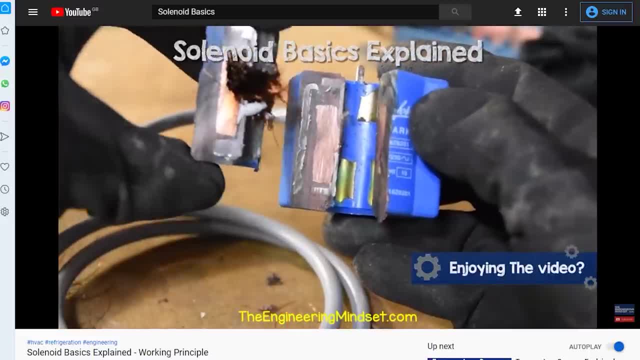 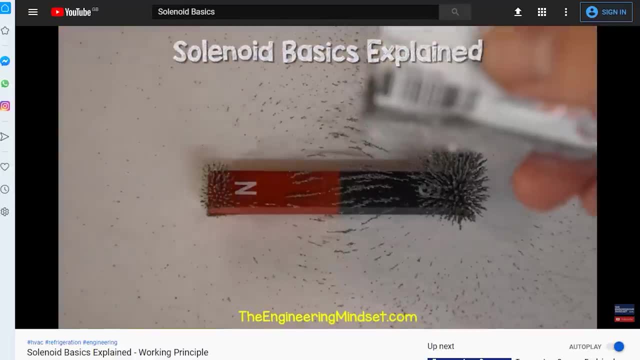 By the way, we have covered how solenoid coils work and even how to make your own solenoid in our previous videos. Do check that out. links can be found in the video description down below. At the end of the electro-magnet we find the armature. This is a small component which 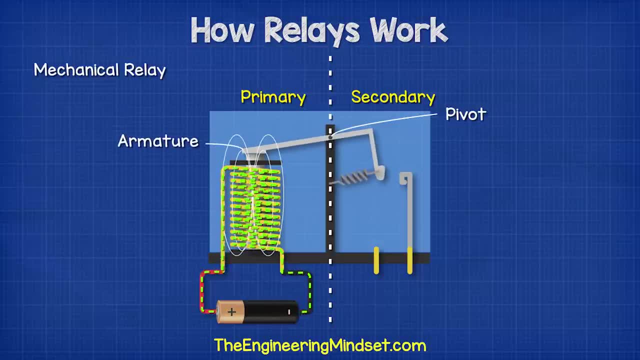 is pivoted. When the electro-magnet energizes, it attracts the armature. When the electro-magnet is de-energized, the armature returns to its original position. A small spring is typically used to achieve this. Connected to the armature is a moveable contactor, And when the armature is attracted to the 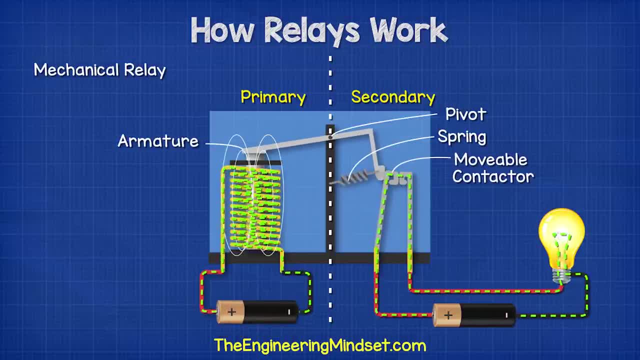 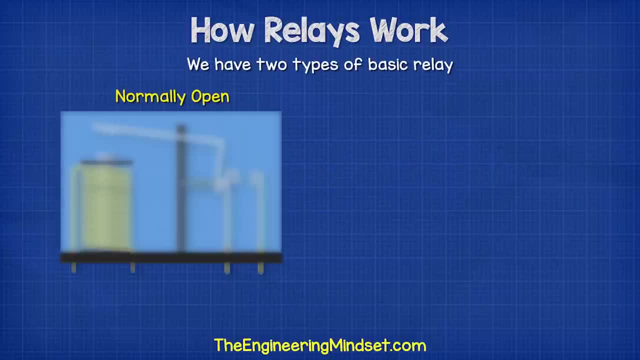 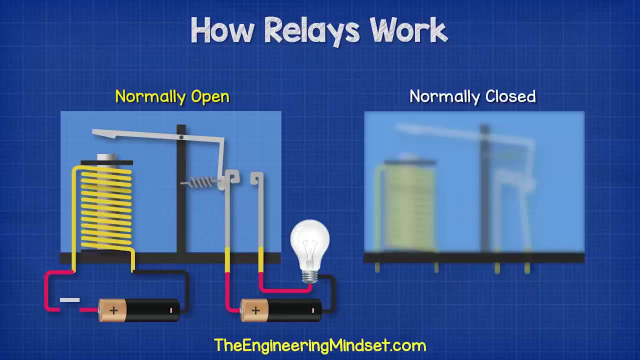 electro-magnet. it closes and completes the circuit. on the secondary side We have two type of basic relays: the normally opened and the normally closed type. There There are other types of relays and we're going to look at these a little later in the video. 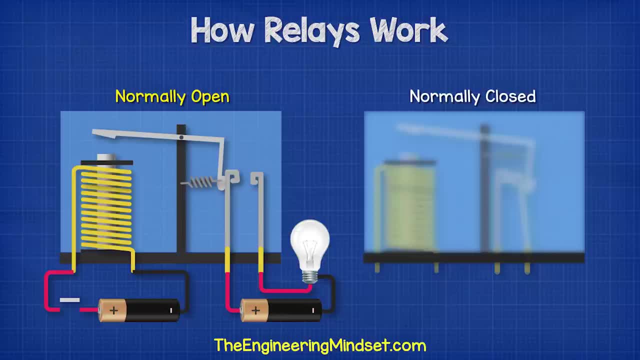 With the normally open type, no electricity flows in the secondary circuit. The load is therefore off. However, when a current is passed through the primary circuit, a magnetic field is induced in the electromagnet. This magnetic field attracts the armature and pulls the movable contactor. 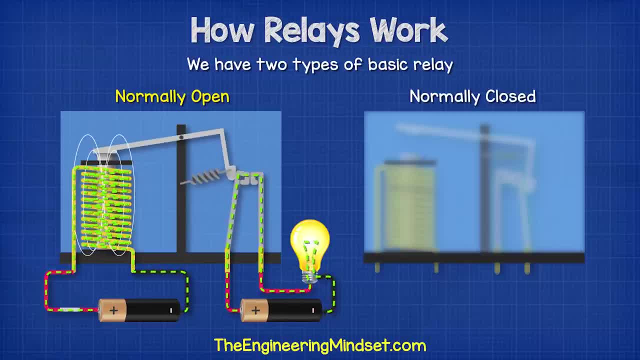 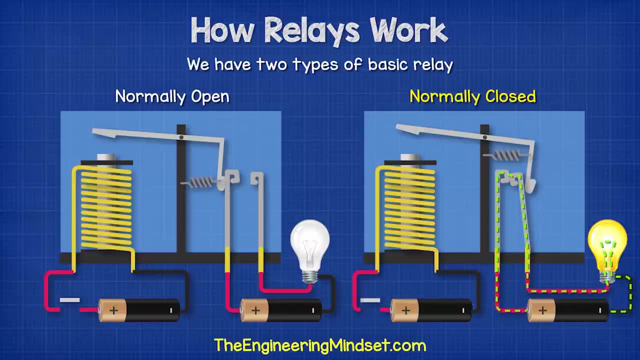 until it touches the terminals of the secondary circuit. This completes the circuit and provides electricity to the load. With the normally closed type, the secondary circuit is normally complete, and so the load is on. When the current is passed through the primary circuit, the electromagnetic field causes the armature to push away. 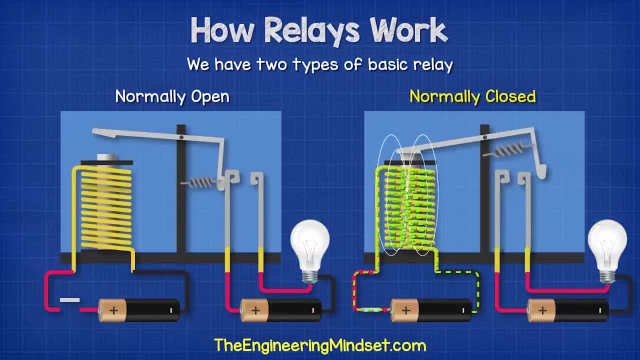 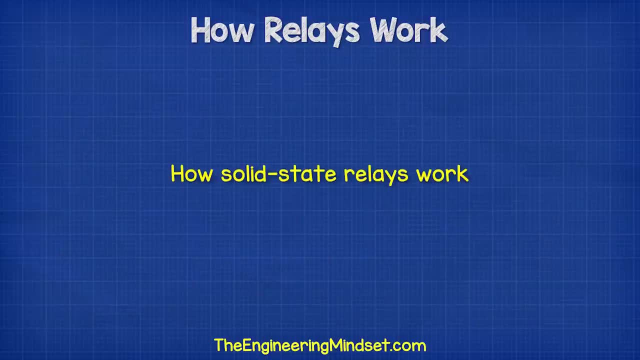 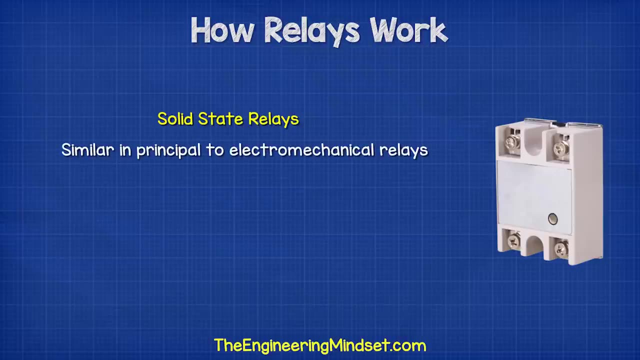 which disconnects the contactor and breaks the circuit. This cuts the supply of electricity to the load. The operation of solid-state relays, or SSRs, is similar in principle, but unlike electromechanical relays, it has no moving parts. 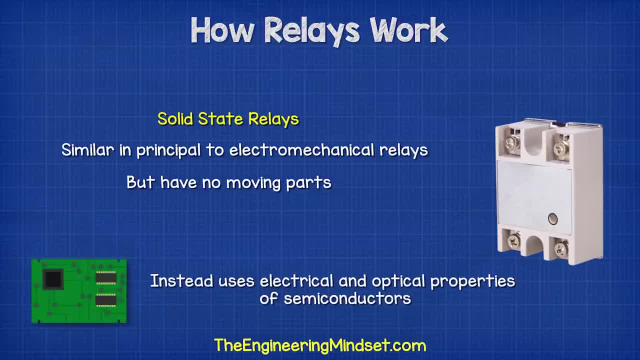 The solid-state relay uses the electrical and optical properties of solid-state semiconductors to perform its input and output isolation, as well as switching functions. With this type of device, we find an LED light on the primary side instead of an electromagnet. 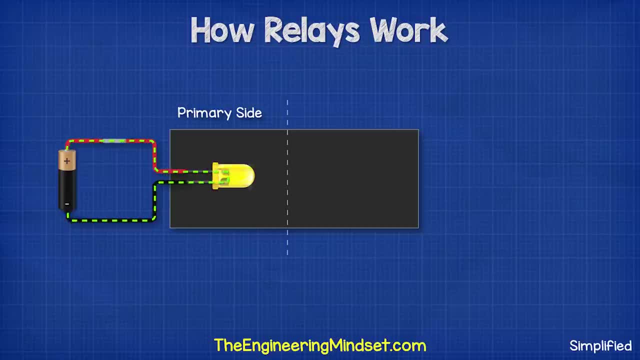 The LED provides optical coupling by shining a beam of light across a gap and into the receiver of an adjacent photosensitive transistor. We control the operation of this type of relay by simply turning the LED on and off. The phototransistor acts something like an insulator. 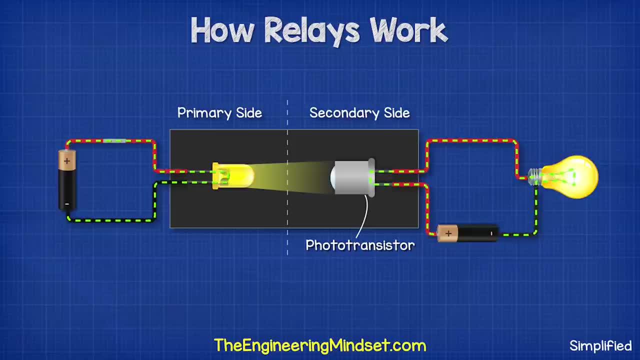 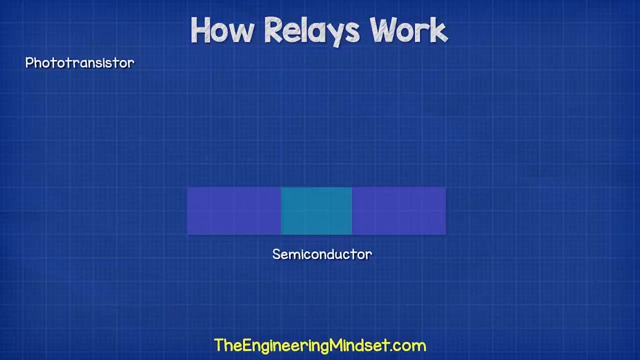 and doesn't allow current to flow unless it's exposed to light. Inside the phototransistor we have different layers of semiconductor materials. There are n-type and p-type, which are sandwiched together. The n-type and p-type are both made from silicon. 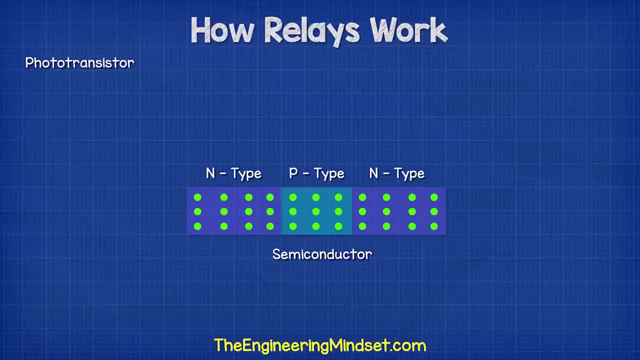 but they have each been mixed with other materials to change their electrical properties. The n-type has been mixed with a material that gives it lots of extra as well as unneeded electrons. These are free to move around to other atoms. The p-type has been mixed with a different material that has fewer electrons. 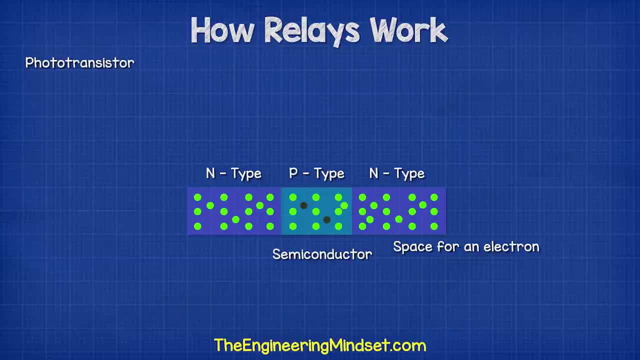 so this side has lots of empty space where electrons can move too. When the materials are joined together, an electrical barrier develops and prevents the electrons from flowing. However, when the LED is turned on, it will emit another particle known as a photon. 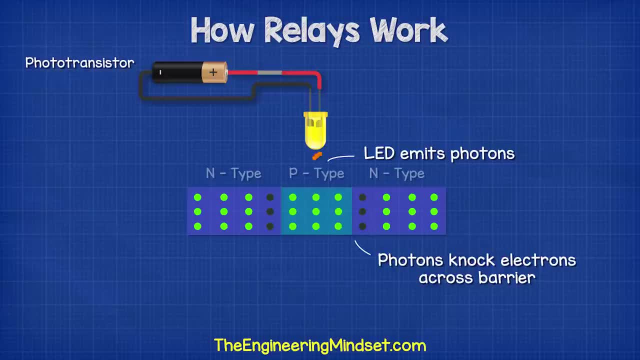 The photon hits the p-type material and knocks the electrons, pushing them across the barrier and into the n-type material. The electrons of the first barrier will now be able to also make the jump, and so a current is generated and the current in the secondary side is developed. 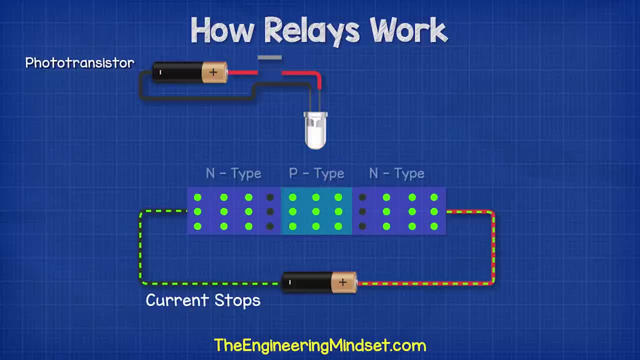 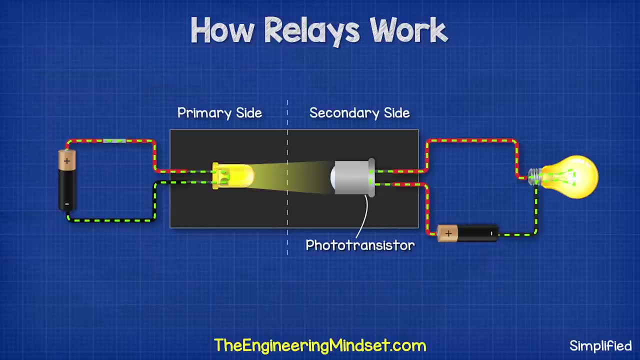 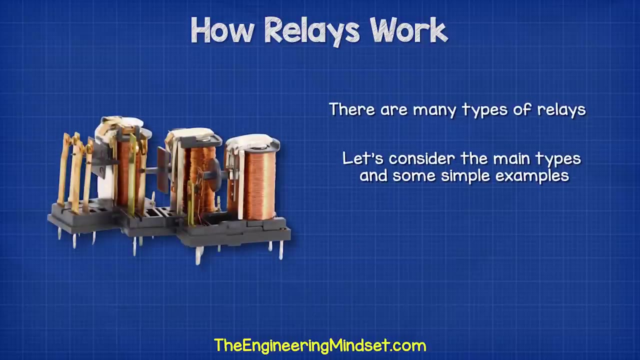 Once the LED is turned off, the photons stop knocking the electrons across the barrier, and so the current in the secondary side stops. So we can control the secondary circuit just by using a beam of light. There are many types of relays, and we're going to now consider a few of the main ones. 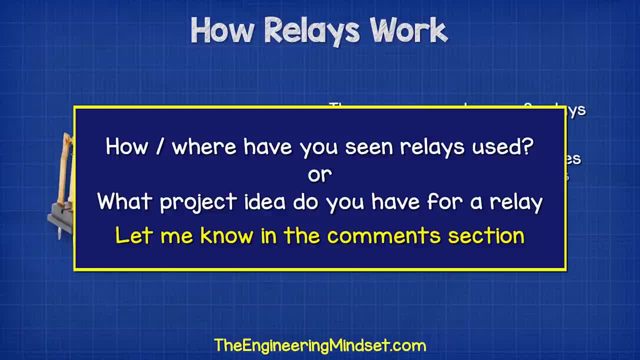 as well as some simple examples of how they are used. Let me know in the comments section where you've seen relays used Or, even better, tell me what ideas you have for their application or any project you're working on where they could be applied. 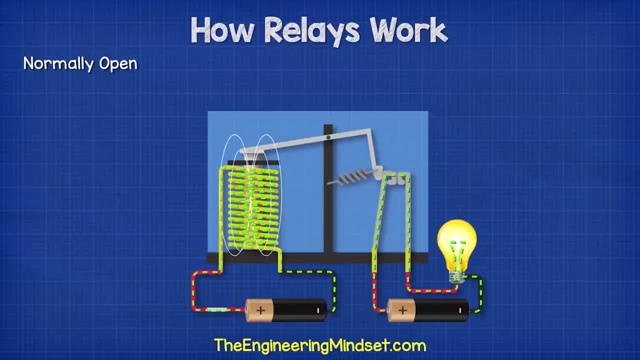 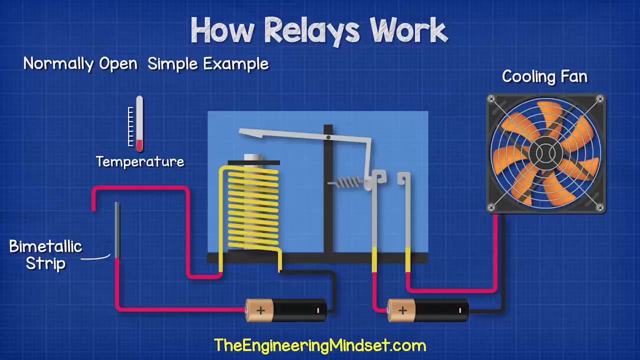 As we have seen earlier in this video, we have the simple normally open relay. This means the load of the secondary side is off until the circuit is complete on the primary. We could use this, for example, to control a fan by using a biometallic strip as a switch on the primary side. 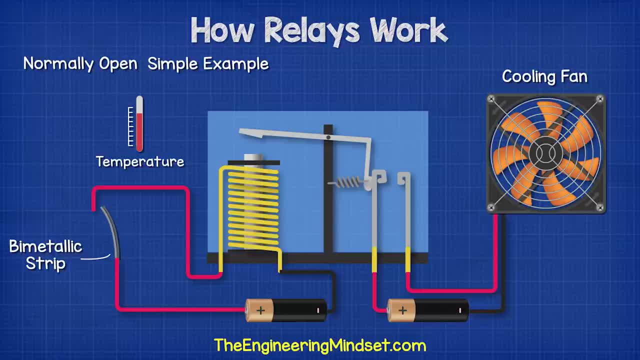 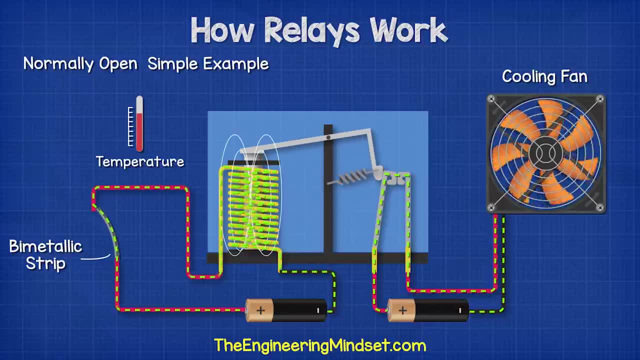 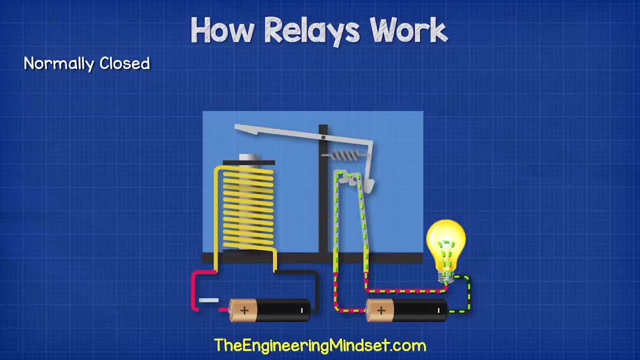 The biometallic strip will bend as it increases in temperature. At a certain temperature it will complete the circuit and turn the fan on to provide some cooling. We also find normally closed relays. This means the load on the secondary side is normally on. 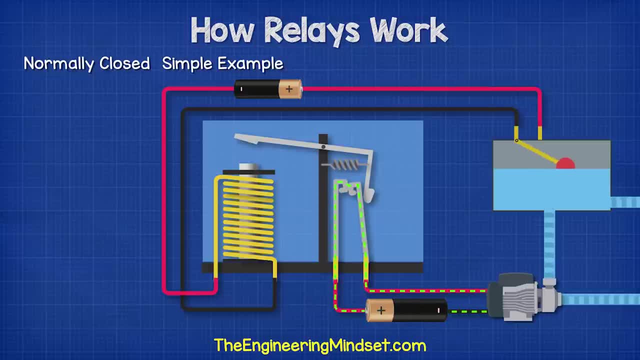 We could, for example, control a simple pump system to maintain a certain water level in the storage tank. When the water level is low, the pump is on, But once it reaches the limit we require, it completes the primary circuit and pulls the contactor away. 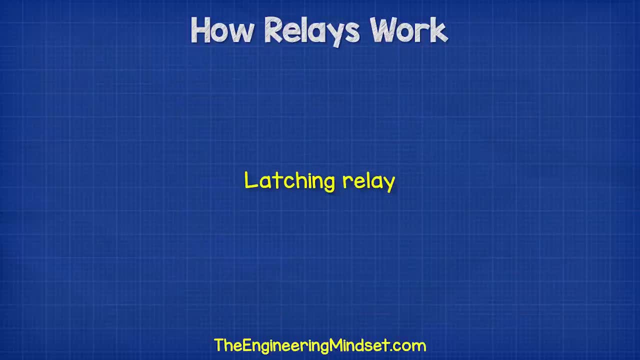 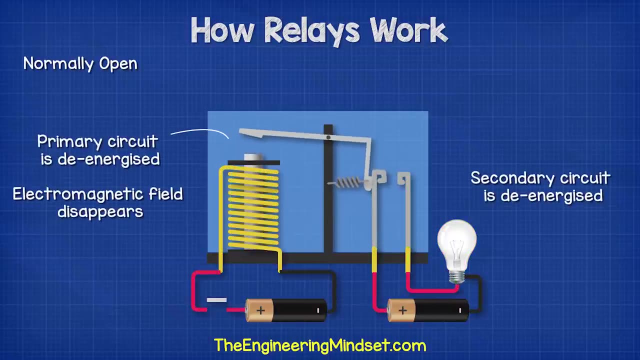 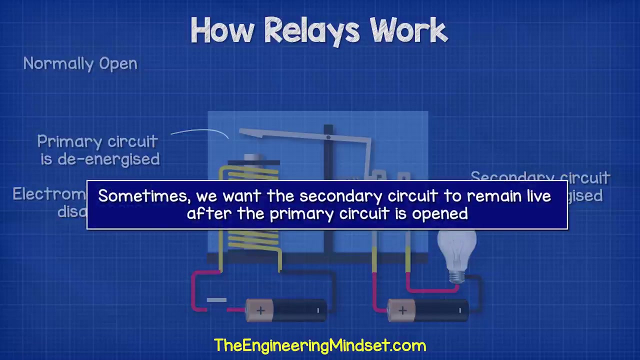 which cuts the power to the pump. In a standard, normally open relay, once the primary circuit is de-energized, the electromagnetic field disappears and the spring pulls the contactor back to its original position. But sometimes we want the secondary circuit to remain live after the primary circuit. 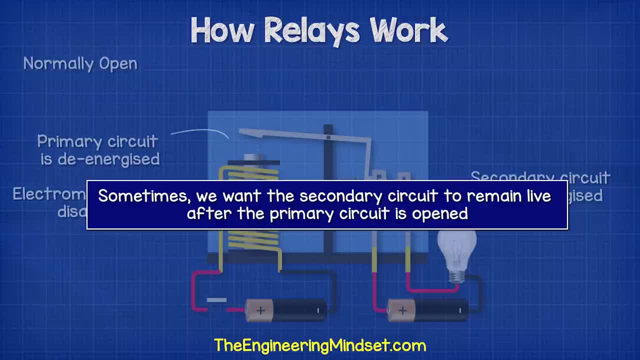 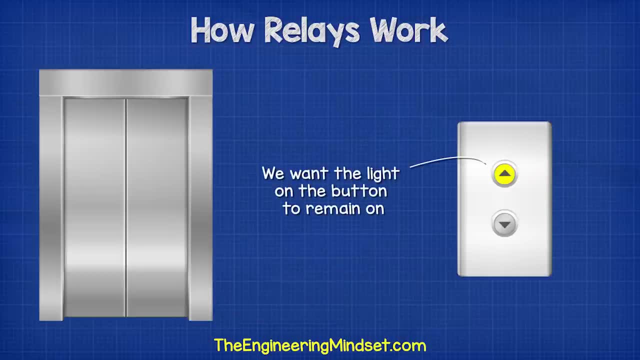 is reopened. For that we can use a latching relay. For example, when we press the call button on an elevator, we want the light on the button to remain on so that the user knows the elevator is coming. So we can use latching relays to do this. 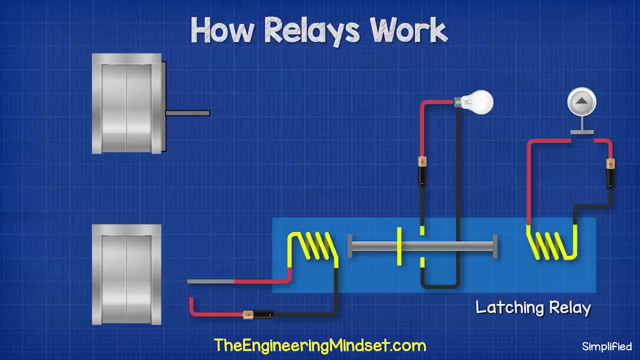 There are many different designs for this type of relay, but in this very simplified example we had three separated circuits and a piston which sits between them. The first circuit is the relay, which is the call button, The second is the lamp and the third is the reset circuit. 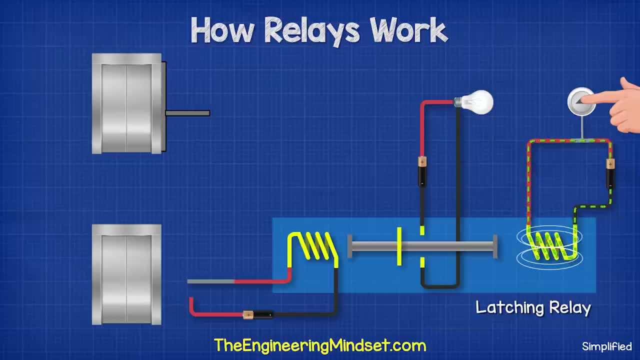 When the call button is pressed, it completes the circuit and powers the electromagnet. This pulls the piston and completes the circuit to turn the lamp on. A signal is also sent to the elevator controller to send the elevator down. The button is released. 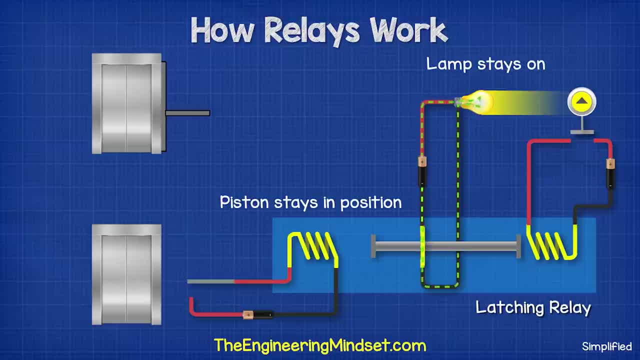 This cuts the power to the initial circuit, but as the piston isn't spring-loaded, it stays in position and the lamp remains on. Once the elevator car reaches the lower floor, it makes contact with the off switch. This powers the second electromagnet. 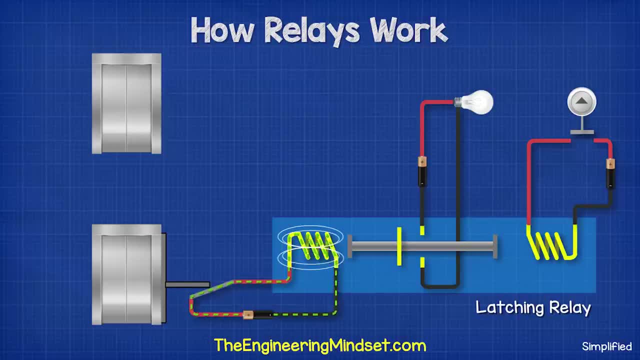 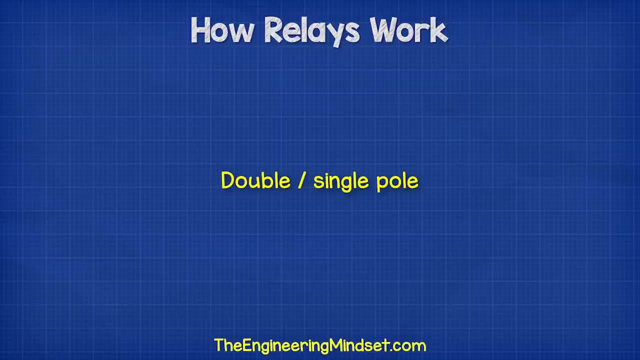 and pulls the piston away, cutting the power to the lamp. Latching relays therefore have the benefit of having positional memory. Once activated, they will remain in their last position without the need for any further input or current. Relays can have single or double poles. 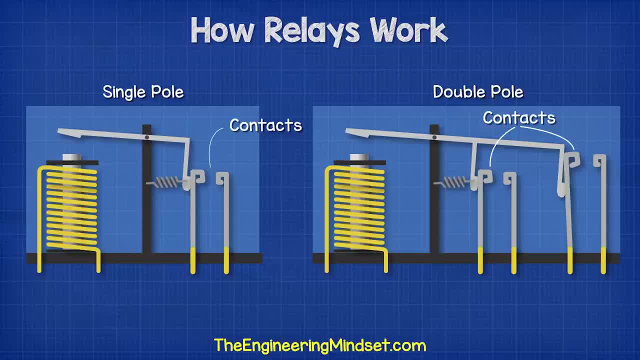 The term pole refers to the number of contacts switched when the relay is energized. This allows more than one secondary circuit to be energized from a primary circuit. We could, for example, use a double pole relay to control a cooling fan as well as a warning light. 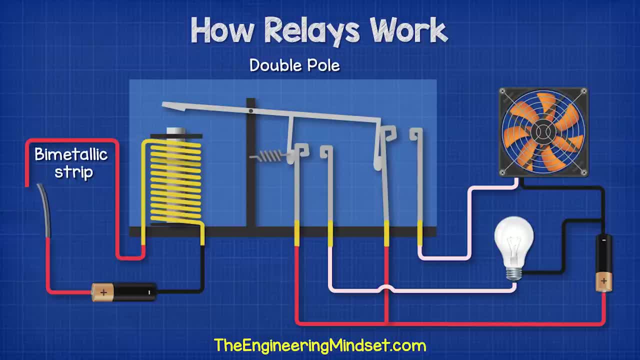 Both the fan and the lamp are normally off, but when the bimetallic strip on the primary circuit gets too hot, it bends to complete the circuit. This creates the electromagnetic field and closes both contactors on the secondary side. This provides power to the cooling fan. 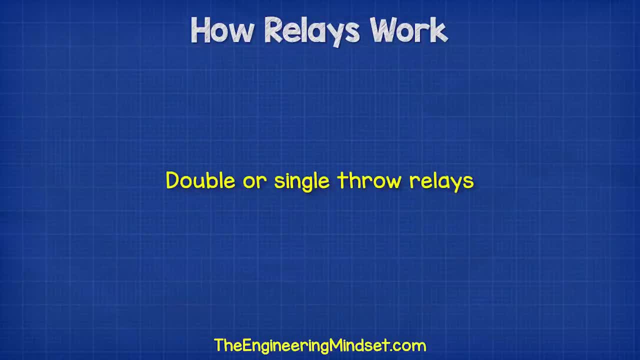 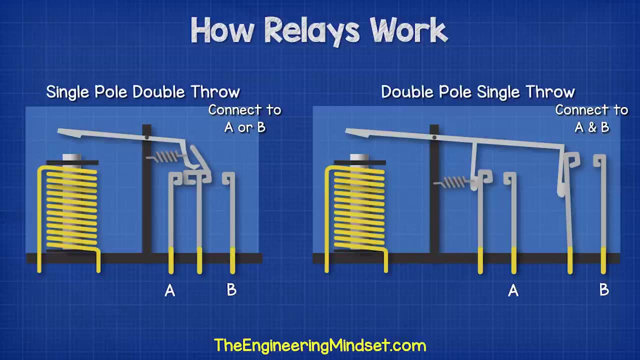 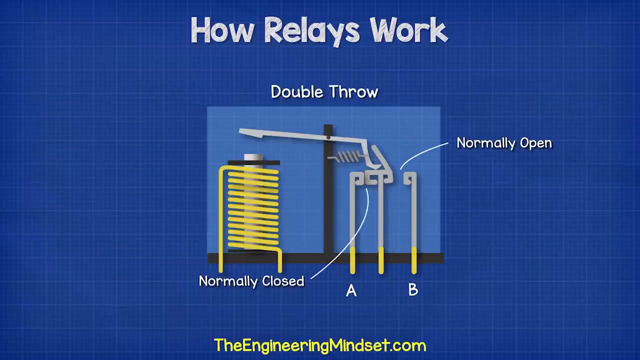 as well as the warning light. When dealing with relays, you'll often hear the term throws. This refers to the number of contacts or connection points. A double throw relay combines a normally open and a normally closed circuit. A double throw relay is also called a changeover relay. 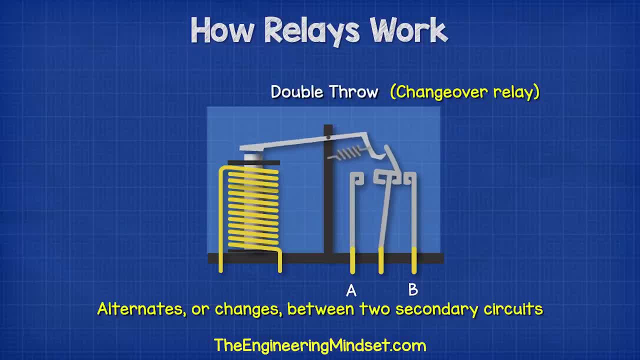 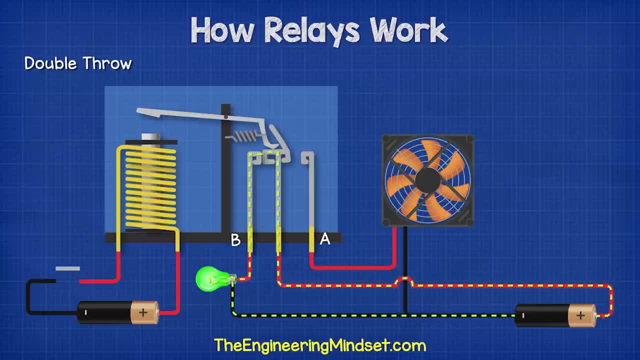 As it alternates or changes between two secondary circuits. In this example, when the primary circuit is open, the spring on the secondary side pulls the contactor to terminal B powering the lamp. The fan remains off because the circuit is not complete. 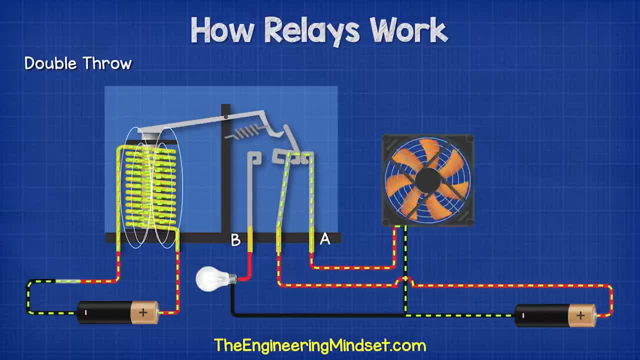 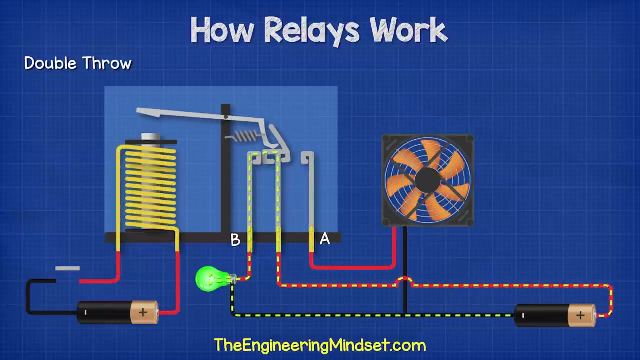 When the primary side is energized, the electromagnet pulls the contactor to terminal A and diverts electricity, this time powering the fan and turning the lamp off. So we can use this type of relay to control different circuits depending on an event. 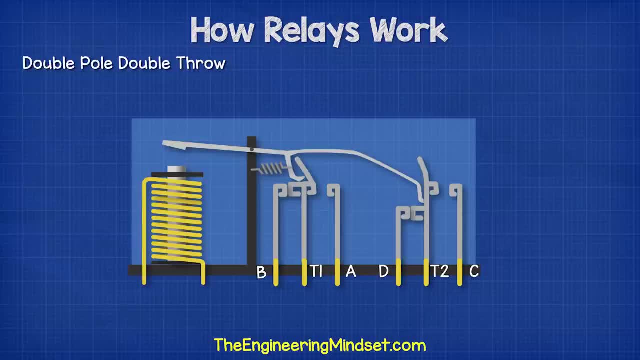 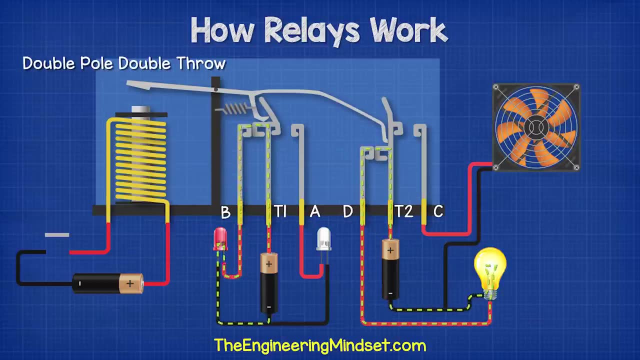 A double pole, double throw relay, or DPDT, is used to control two states on two separate circuits. Here we can see a DPDT relay When the primary circuit is not complete. terminals T1 and T2 are connected to terminals B and D respectively.